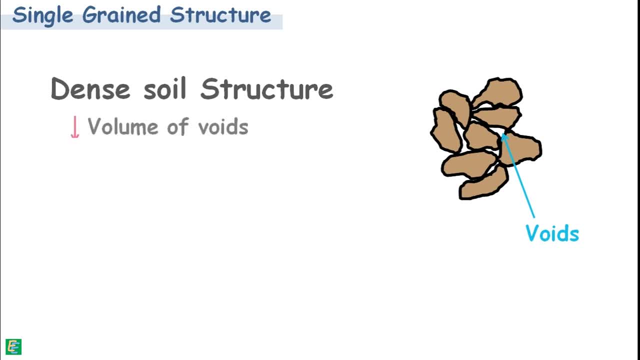 denser is the structure, As volume of voids is less, lower will be its void ratio and lower will be its permeability. Dense soils have high shear strength and low compressibility, which makes them more preferable for engineering purposes, While soil particles which are loosely packed, leaving large void spaces between them, make 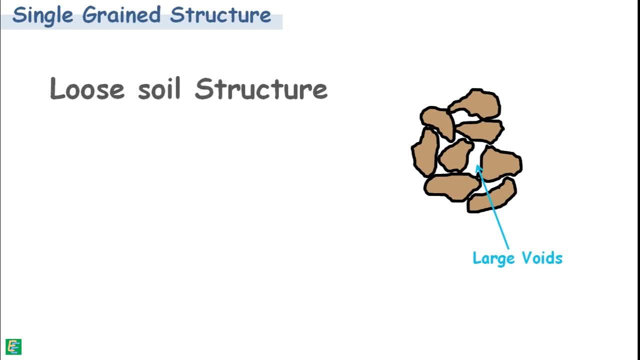 up loose soil structure. Loose soil structure has large volume of voids, hence they have high void ratio and high permeability. But they are unstable. When loose soils are subjected to vibrations, their particles move and acquire a more stable position and form a denser state. 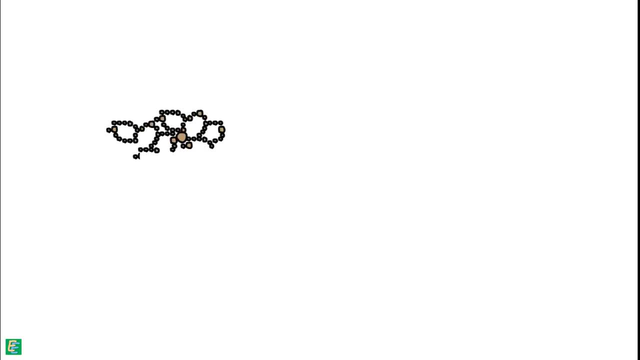 Sometimes smaller soil particles of silt size when depositing join with one another and form a bridge like structure. They contain very large voids between these bridges and make the soil very loose in nature. Such a formed structure is called honeycomb structure. As soil in a honeycomb structure is loose, they can support load only under static condition. 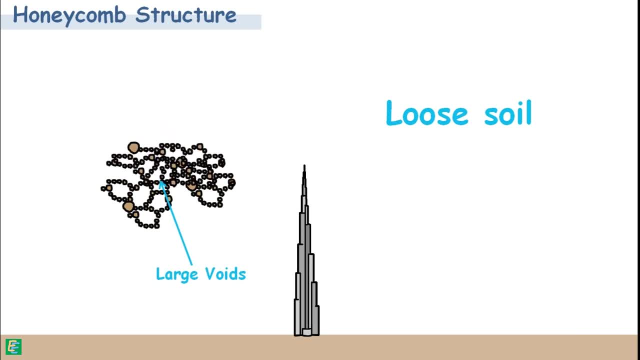 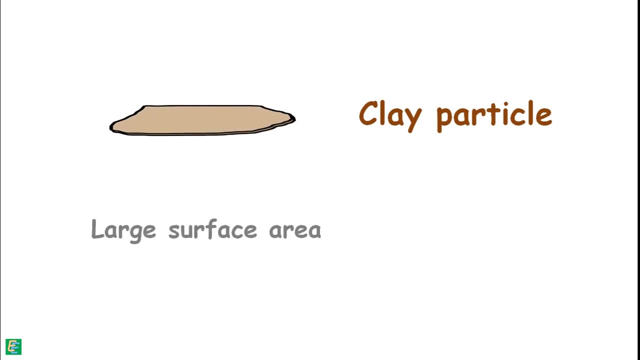 When they are subjected to vibration or shock, they form a denser state. The structure collapses, large deformations take place and the soil achieves a relatively denser state. Clay particles are very small, flaky in shape and they have a large surface area. and because 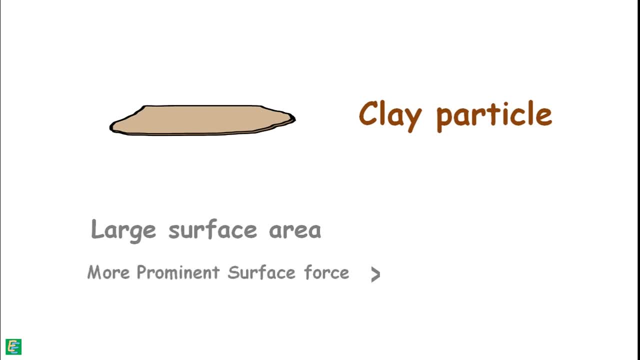 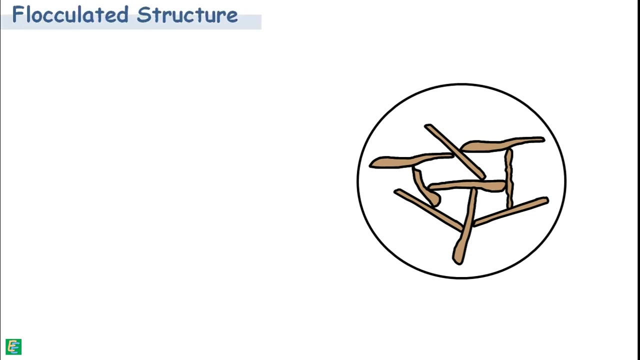 of that their surface forces are more prominent in them than gravitation force. These particles have negative charge on the surface and positive charge on the edges. They combine each other by joining negative surface of the particle to the positive edge of the other. This way they form a soil structure which is called flocculated structure. 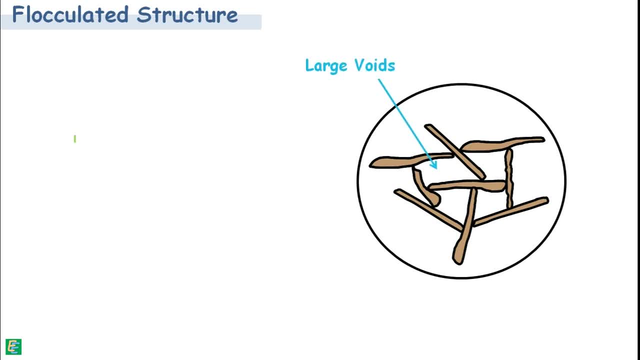 We can see. soils with flocculated structure have large amount of voids, So their void ratio is high. These soils are less sensitive to vibrations as they formed a strong electrical bond. 4. Clay Soil. Clay particles are remoulded, their flocculated structure changes and particles change their